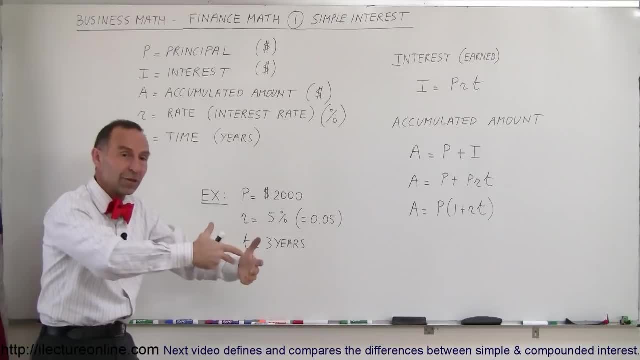 but there was a time where we earned a fair amount of money in the bank. You want to put in the bank to earn some interest. That's your principal. That's your principal. investment. Interest is the amount of money that you get in return for that. The bank will pay you money. 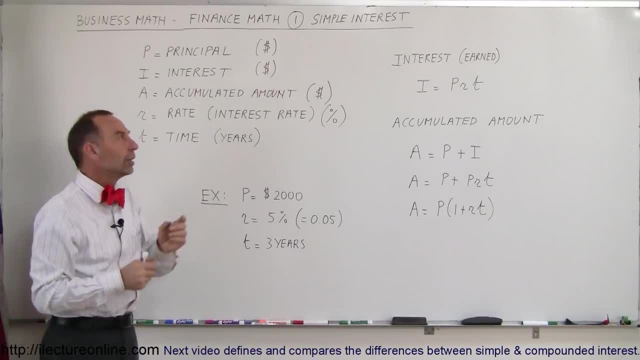 and that's called interest. You will earn interest, And so the unit for interest is dollars, Not to be confused with the interest rate. We'll get to that in just a moment. A stands for accumulated amount. The total amount that you end up with will be the initial. 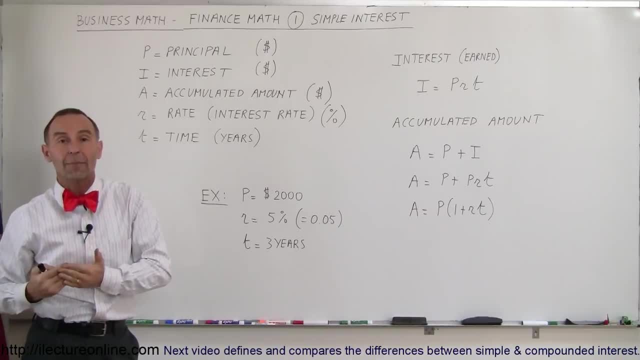 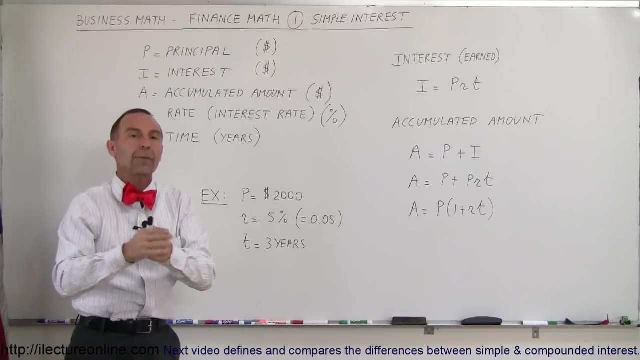 principle you put in the bank, plus whatever interest you put in the bank you earn on top of that. so the two combined will form the accumulated amount. so the more interest you earn, the bigger the accumulated amount which is added to the initial principal investment that you made. next is called 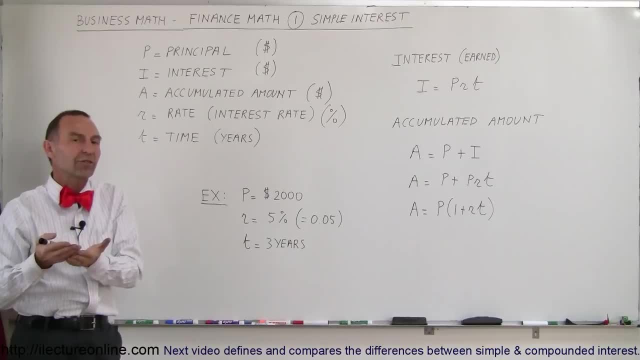 our for rate. that's called the interest rate, usually expressed in percent or in decimal, so that's how fast you'll be accumulating interest. it's based upon the rate and, of course, about how much you invest as well. but if the rate is high, helium you'll get more interest is: erase this low, you'll get less interest. 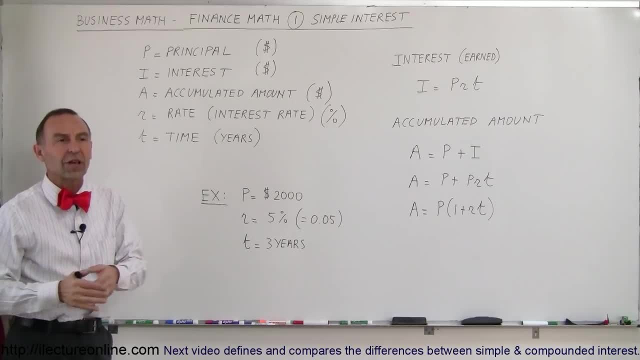 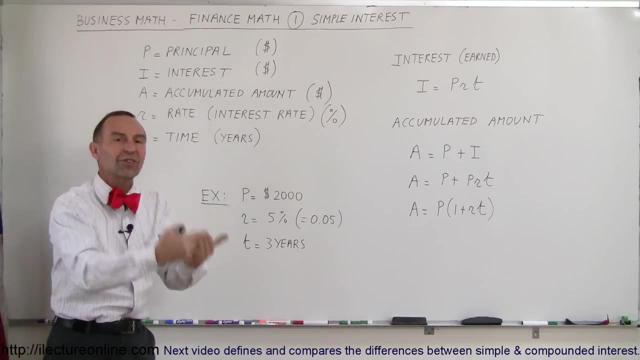 so usually it's like one percent or two percent or three percent. so for every year that you put your money in the bank, they will give you some money back. and else, in terms of what percent of your principal will they pay you? and that's called the rate, and finally, the time and use. it's expressed in years. how? 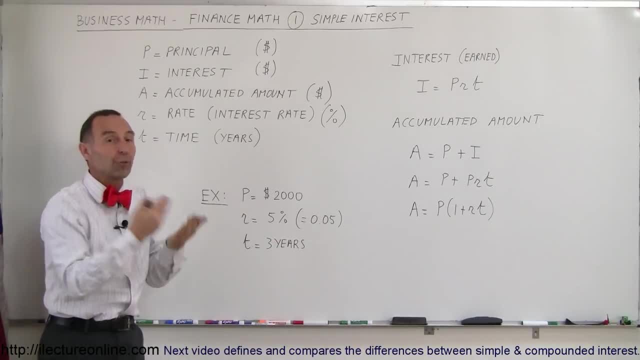 long will you put your investment in the bank? if you put it in for one year, you'll earn interest for a year. if you put in for two years, you'll interest for two years years. Simple interest means that you put it in and then at the end of the period they will give. 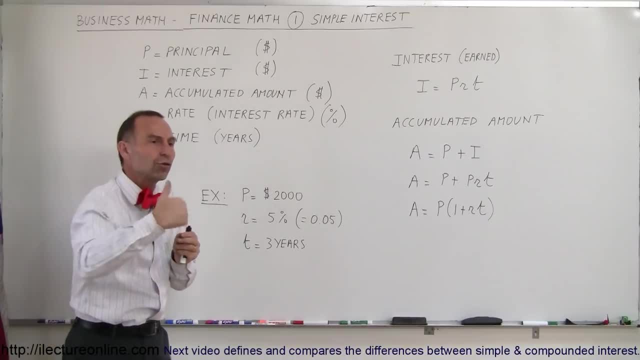 you the interest and they will not pay you interest on the interest that you're earning along the way. That's the difference between simple interest and compounded interest. So if you leave it in for three years, after three years they'll say: well, you turn in, you put in. 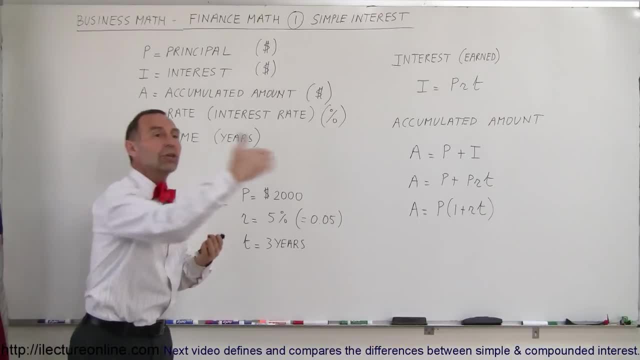 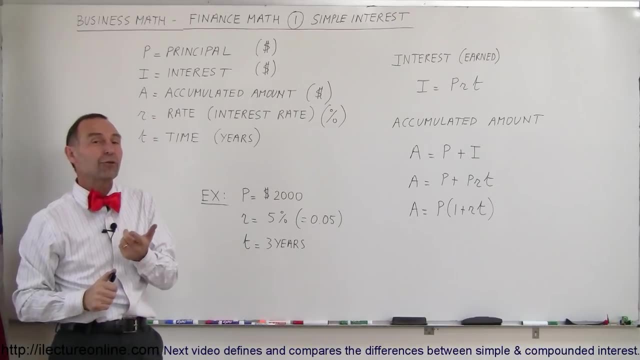 $1,000 in the bank, you get this rate and after three years you'll get this much money and they don't pay you on the interest that you're earning. while the money is in the bank It's not as lucrative. so therefore the compounded interest rate is the one that's most used most of the 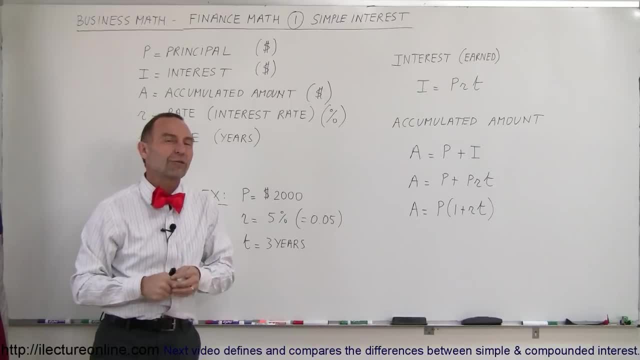 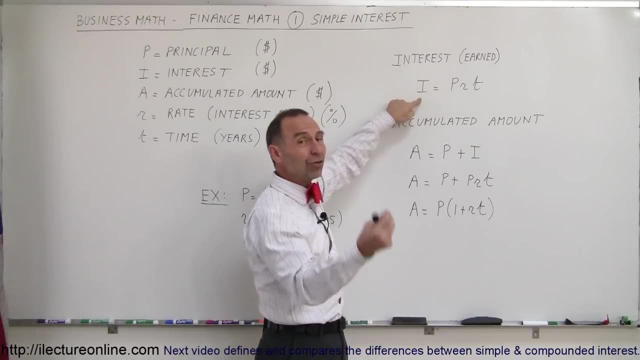 time used because it is a more advantageous way of earning money, and we'll get to that in a later video. So definition of interest: mathematically the amount of money that you get back for investing your principal. it's equal to the principal you invest, times the rate at which it's invested at. 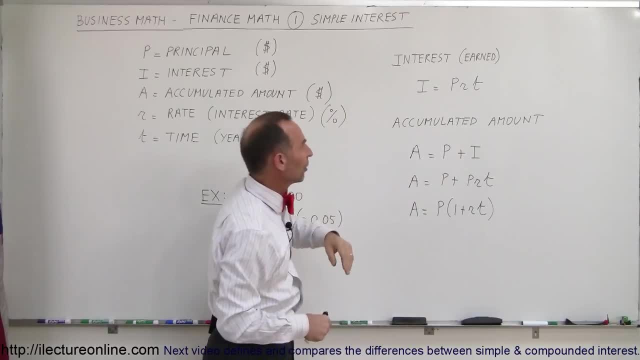 times the amount of time that you leave it in the bank. So it's principal times rate. times time will give you interest earned and the result is in dollars. The accumulated amount is the amount that you end up with at the end, which is equal to the. 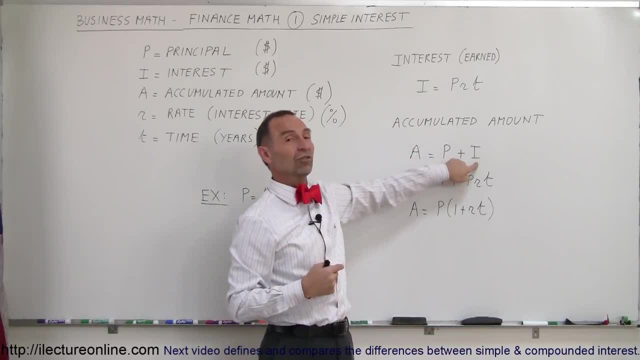 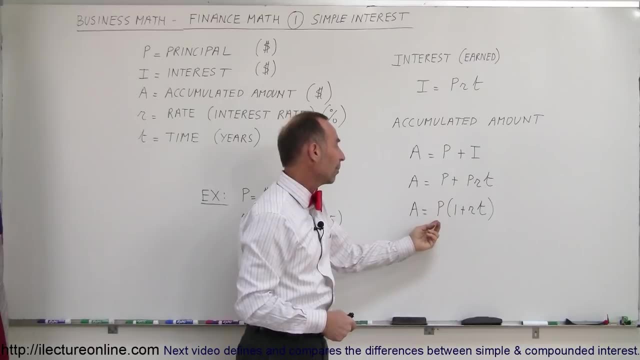 principal you invested, which of course you'll get back, plus any interest that you earned. And since the interest that we earned is going to be equal to PRT from our definition, we can then factor out a P, the principal, so that means the amount. the accumulated amount will be the. 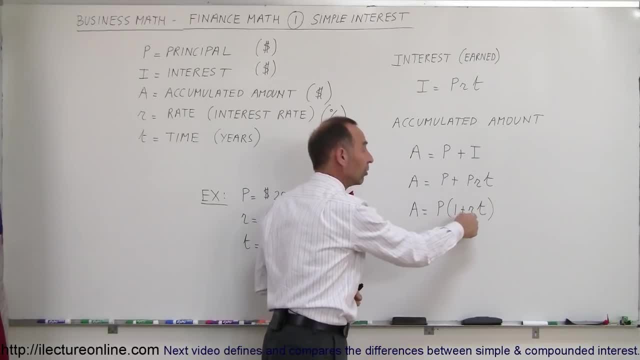 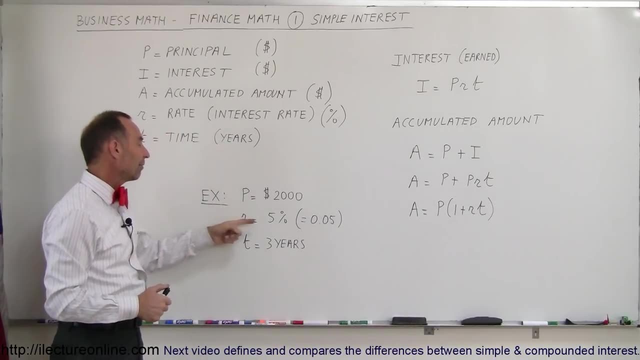 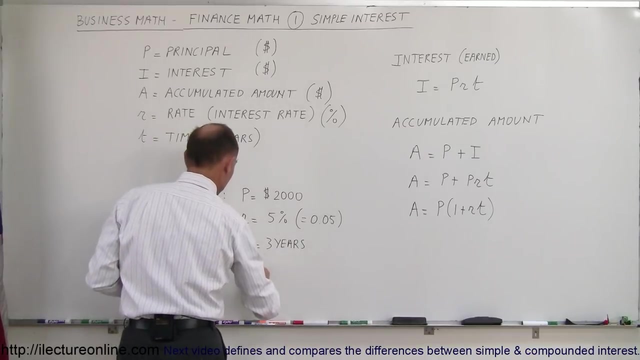 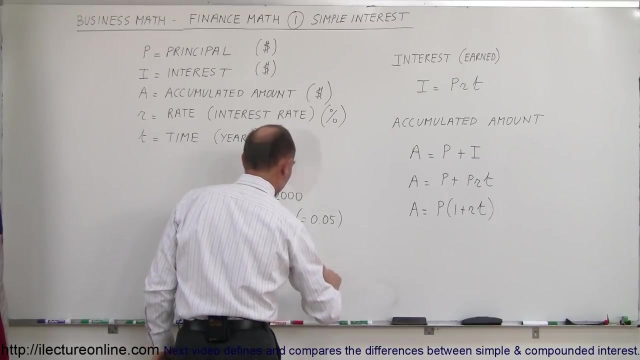 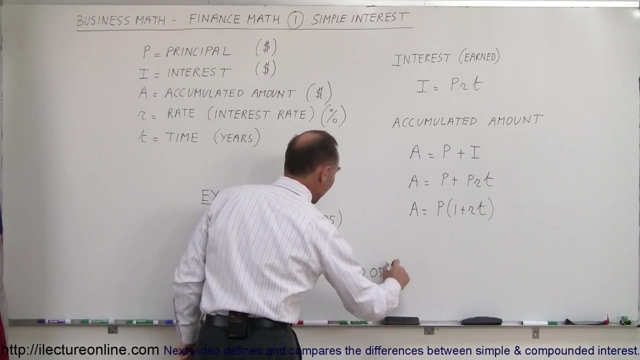 principal times the quantity, one for the initial principal, plus the rate times the time. All right, so here's an example Here. let's say that we're going to invest $2,000 at 5% interest rate and we'll do it for three years. but it's simple interest, which means that the interest that you'll earn I, which is equal to the principal times the rate, times the time, which is going to be equal to $2,000, times the rate which is 5%, so that will be 0.05, times the time, which is three years. 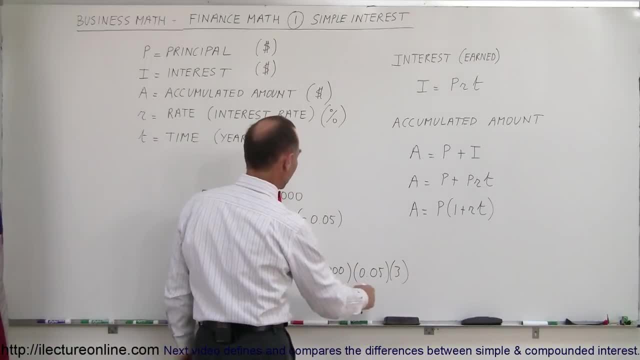 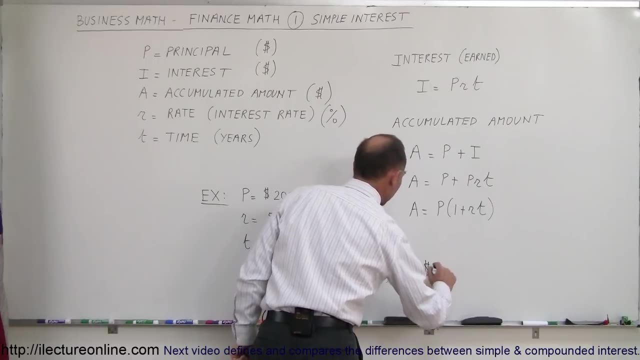 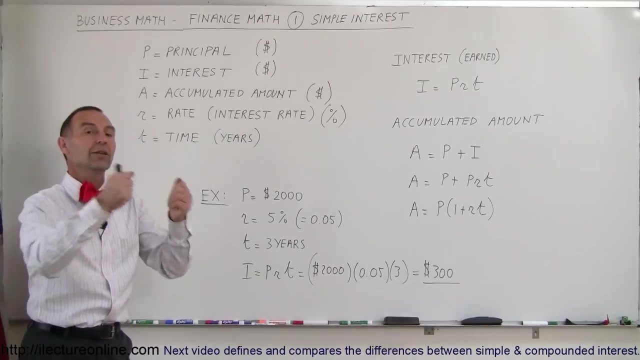 So what is the total amount? Let's see here: 5% on $2,000 is that would be $100 times three. so that would earn you $300 after three years. After three years you would get your $2000 back. they will pay an additional. 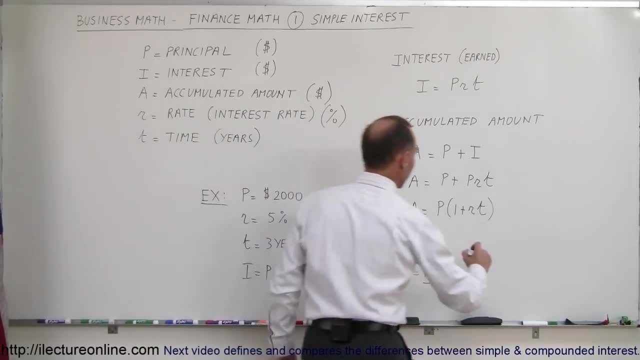 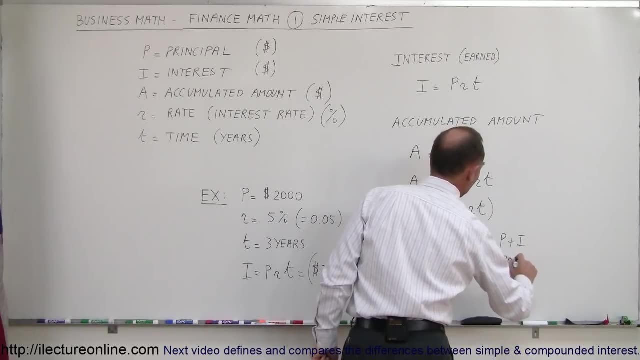 $300.. So what would be the accumulated amount? So, since the accumulated amount is equal to the principal plus interest, so in this case the principal will be $2,000, that's the initial investment plus the three hundred dollars that you earn on interest after three years. 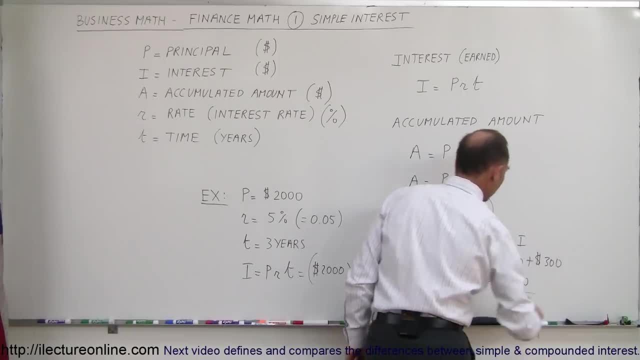 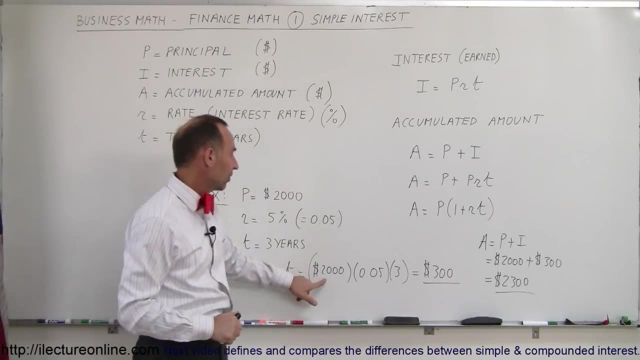 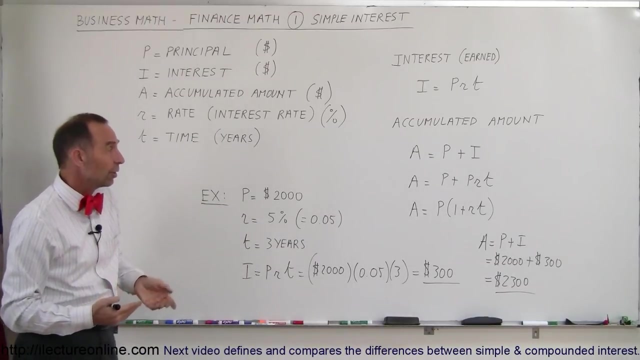 which equal to two thousand three hundred dollars, which will be the accumulated amount that you'll end up with after three years. Okay, so, quick check: that's ten. that's a hundred times three, three hundred. that looks correct. So that's the concept of simple interest. It's very straightforward.